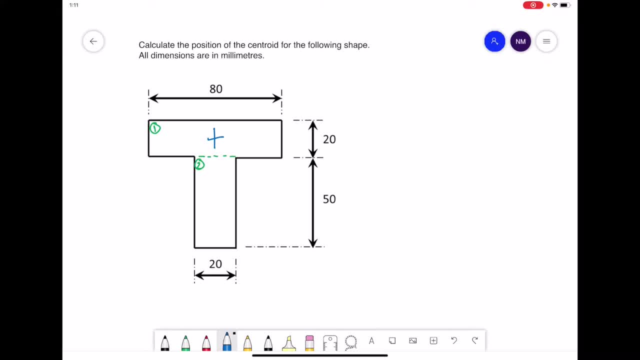 The centre for each individual rectangle is half the length along and half the height up, So drawing in a centre for each of the rectangles. What we need to do is to be able to specify the centre of or specify the location of these centres relative to one reference point. 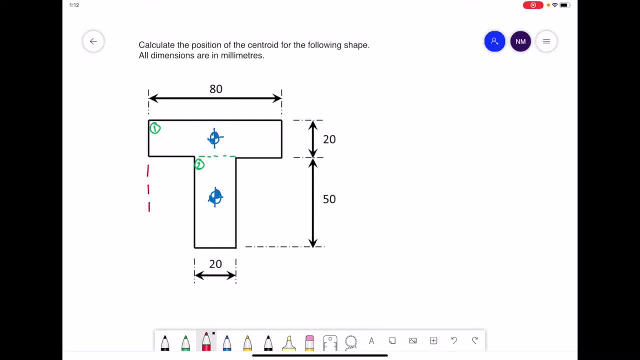 The reference point that is used is the lower, most left most point that we have on the shape, And in this case it's our location down here in the bottom left hand corner. Sometimes it will be a point that's actually on the shape. 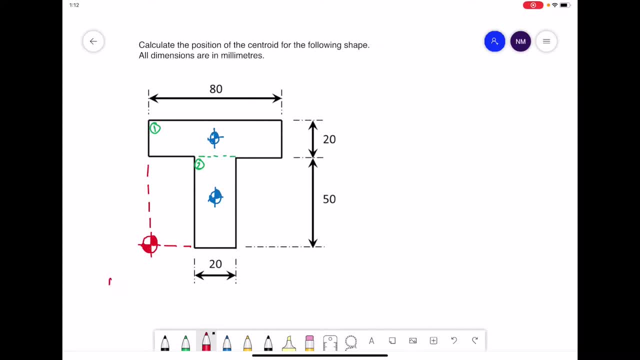 In this example, it's a point that is in free space. Our reference point is like the origin. on a graph, Co-ordinates are 0, 0 and from this reference point we're going to measure the location of the centre for each of the two rectangles that we have in this case. 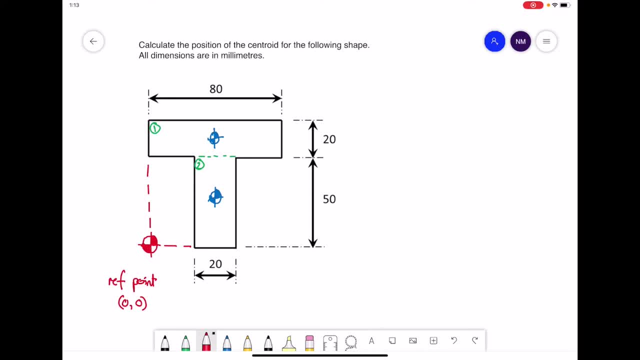 To decide. I'm going to write down the co-ordinates of the centre for each of the rectangles To do that, starting with rectangle 1.. It will be 40.. 40mm across And we'll have a height of 50 plus 10.. 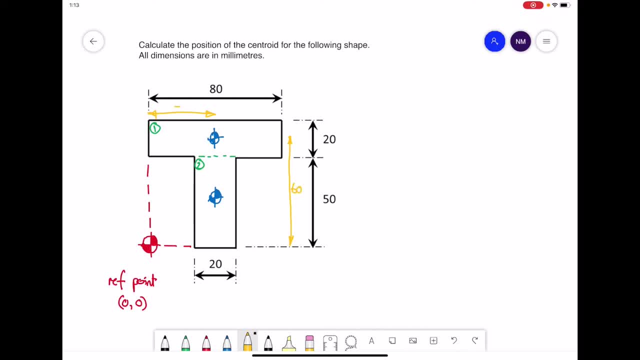 And that will give us 60.. So 40 across and 60. Write that to the side as a co-ordinate: 40 across, 60. up For the second rectangle. again we have to measure the distance across. 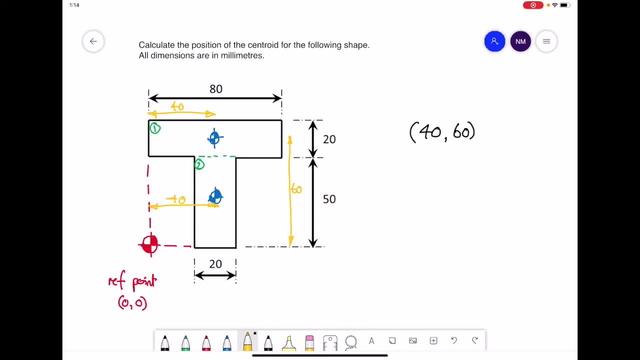 40mm, and the height in this case will be 25.. Writing that down as a co-ordinate: 40, 25.. Underneath each of these sets of co-ordinates, I'm going to write down the variables x1,. 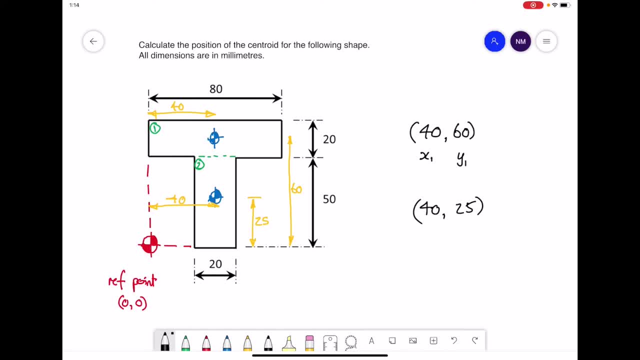 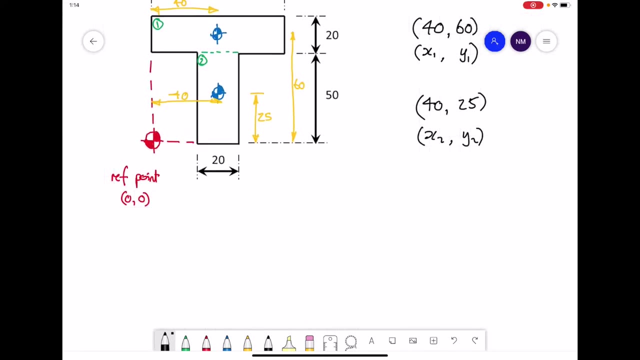 y1, because these pertain to rectangle 1.. And on the second set, x2, y2, because they pertain to the second rectangle. Now the formula we need to work out the position of the centroid is For x bar sigma ax, over sigma a. 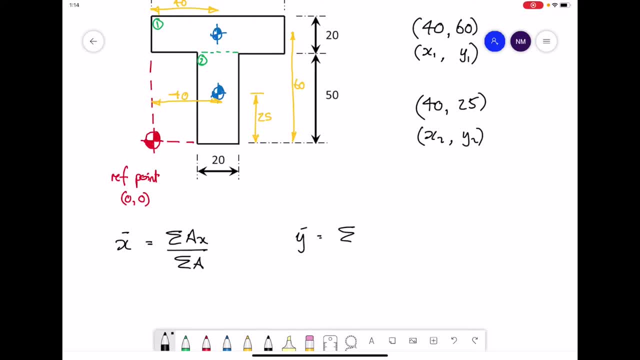 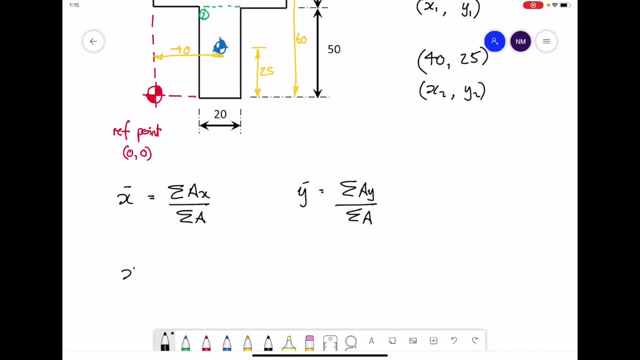 And for y bar it's sigma ay over sigma a, Taking the first of these two formula, sigma means sum of. So we take the area of the individual rectangle, Multiply it by its co-ordinate 40.. Co-ordinate distance. 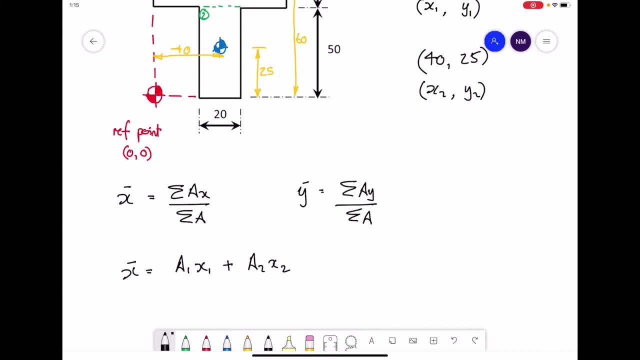 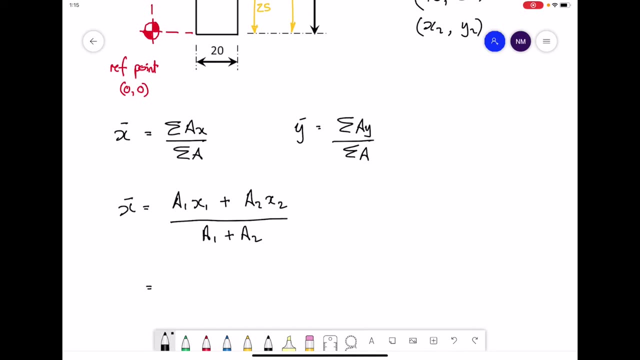 Do that for all the rectangles you have in your shape. In this case there's only two rectangles. Then divide it by the total cross-sectional area, Area 1 plus area 2.. Now putting some values into our equation. First, rectangle 80 by 20.. 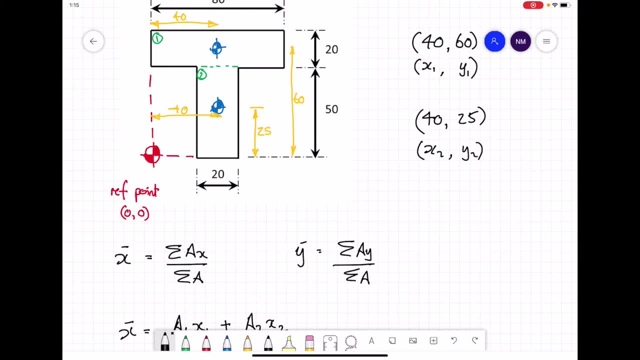 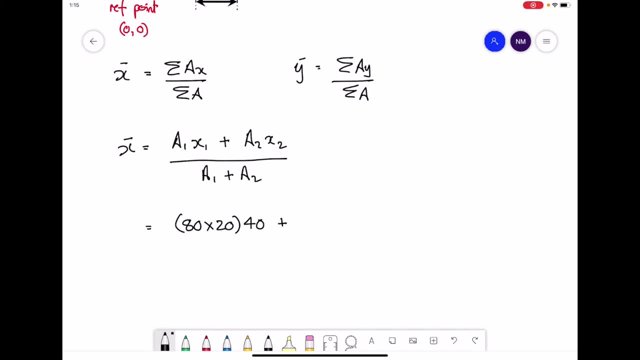 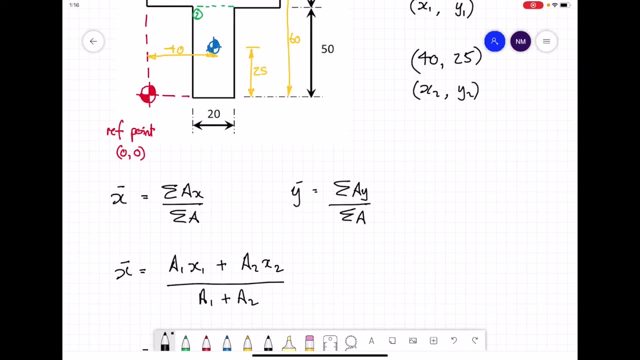 And the x1 value we can see Is a value of 40.. Goes into our equation For the second rectangle. It will be 20 across and 50 tall And its x2 value, you can see, Is a value of 40.. 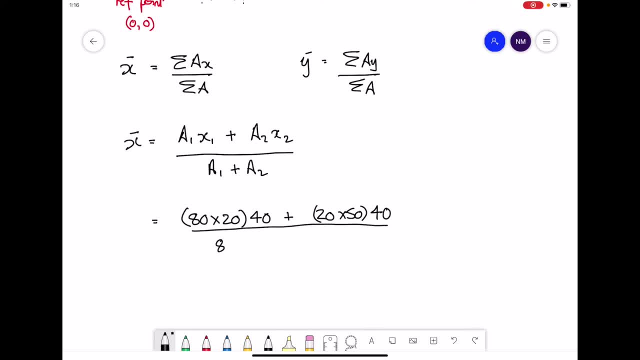 Divide that by the total cross-sectional area, 80 by 20.. Plus 20 by 50. Work that out with your calculator- You get 104,000.. Divided by 2,600. And that gives you a value of 40 mils.